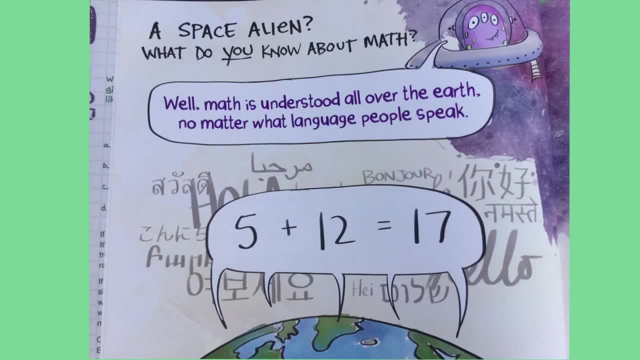 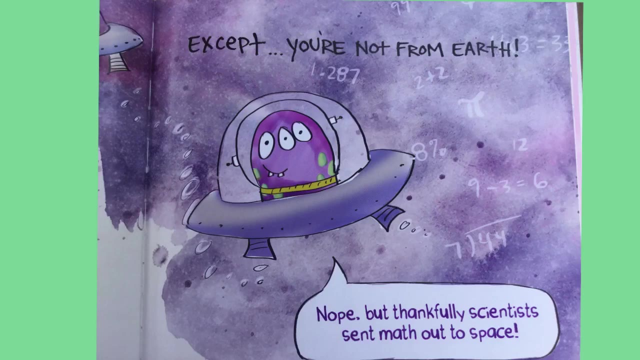 A space alien. What do you know about math? Well, math is understood all over the Earth, no matter what language people speak, Except you're not from Earth, Nope. but thankfully scientists sent math out to space. Scientists took examples of life. 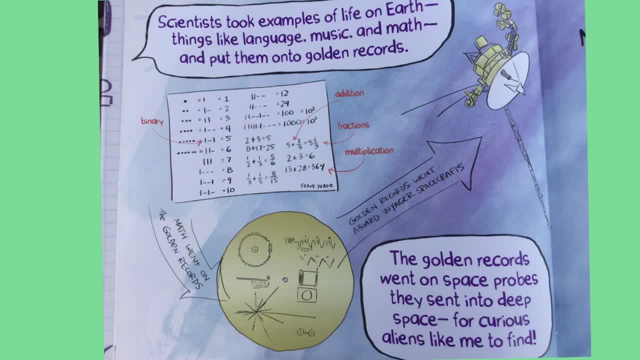 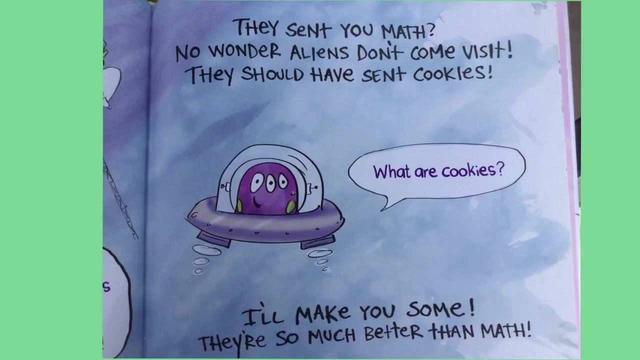 Life on Earth, things like language, music and math, and put them onto golden records. The golden records went on space probes. they sent into deep space for curious aliens like me to find. They sent you math. No wonder aliens don't come visit. 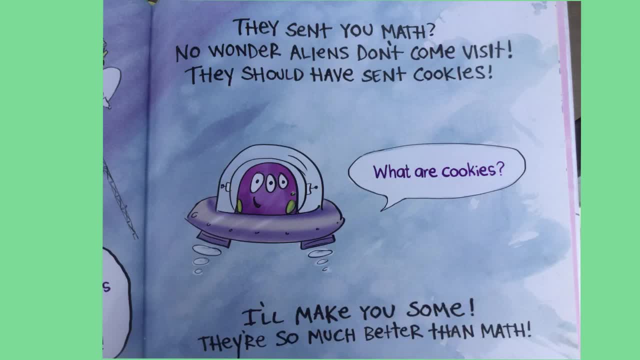 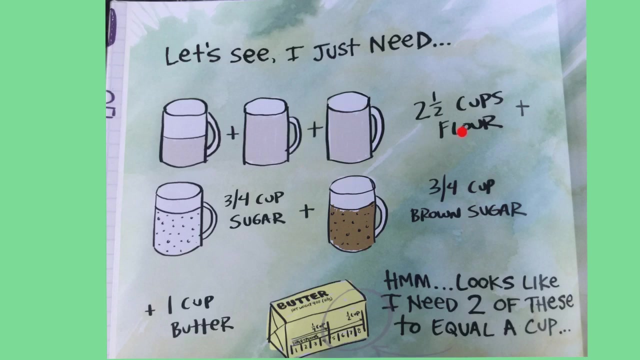 They should have sent cookies. What are cookies? I'll make you some. They're so much better than math. Let's see, I just need two and a half cups of flour and three-fourths cup sugar and three-fourths cup brown sugar and one cup butter. 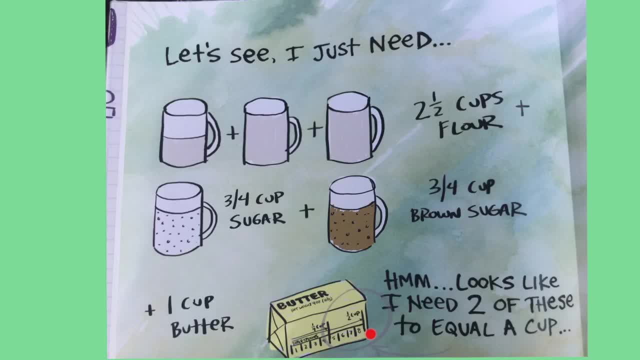 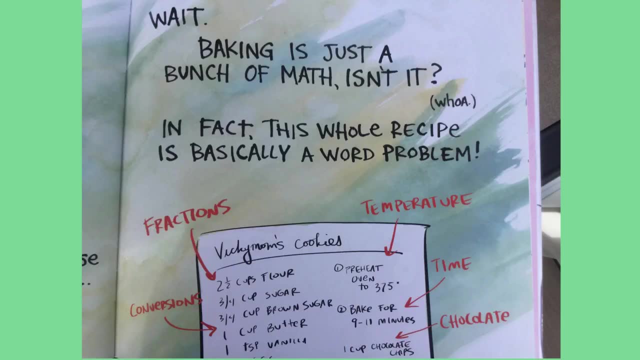 Hmm, looks like I need two of these to equal a cup. Wait, baking is just a bunch of math, isn't it? Whoa? In fact, this whole recipe is basically a word problem. It has fractions, temperature conversions, time, chocolate. 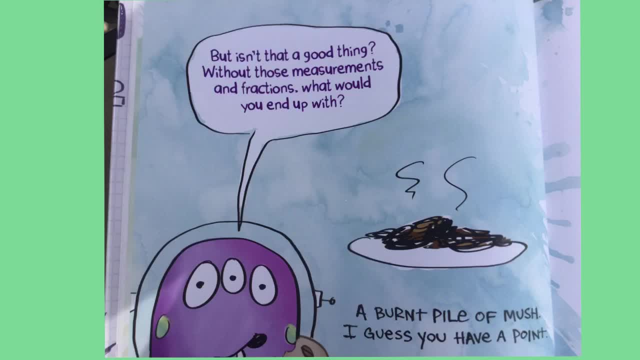 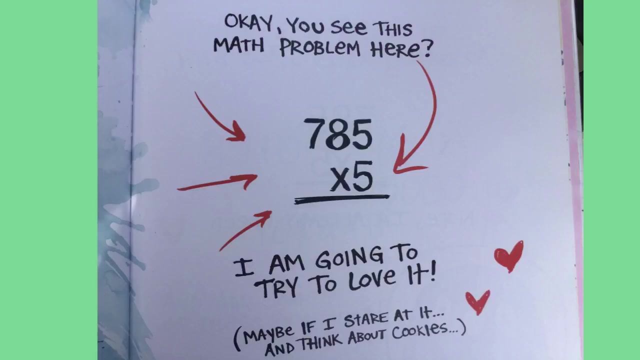 But isn't that a good thing? Without those measurements and fractions, what would you end up with? A burnt pile of mush. I guess you have a point. Okay, you see this math problem here Here: 785 times 5.. 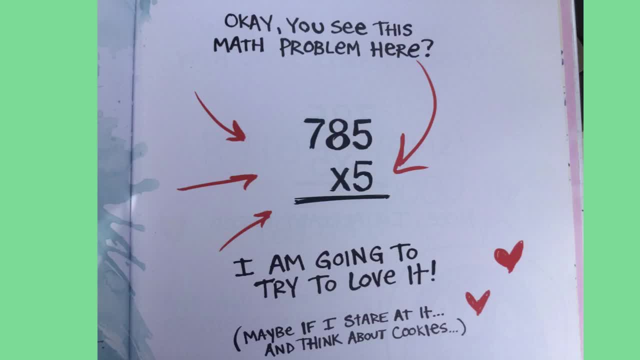 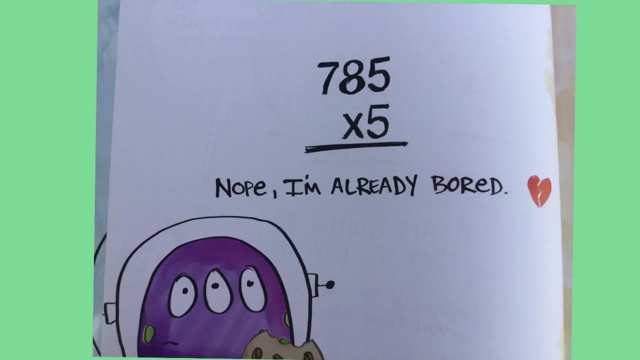 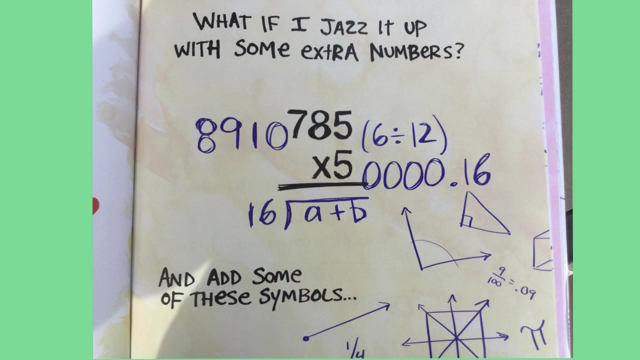 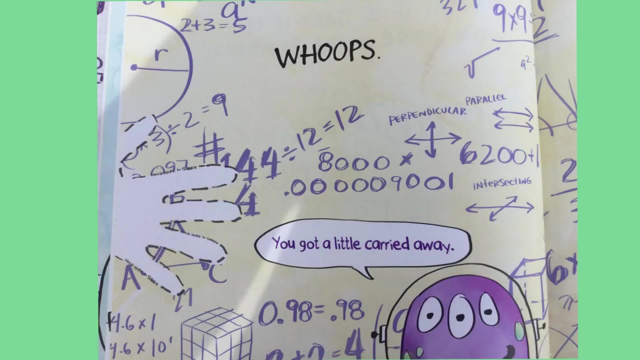 I'm going to try to love it, Maybe if I stare at it and think about cookies. Nope, I'm already bored. What if I jazz it up with some of these extra numbers, Yes- And add some of these symbols? Whoops. 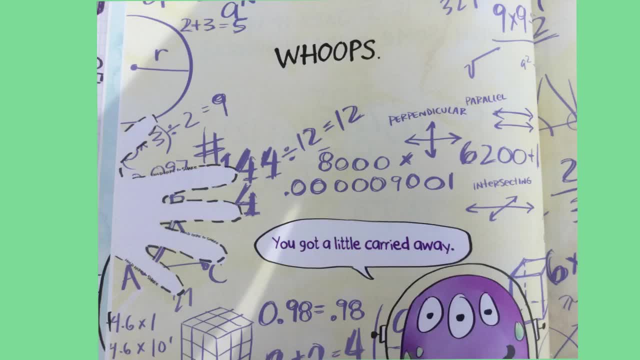 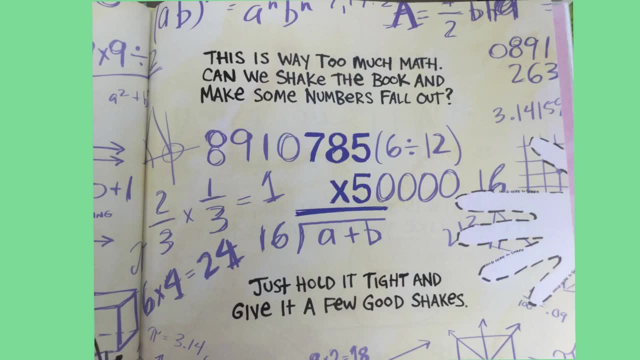 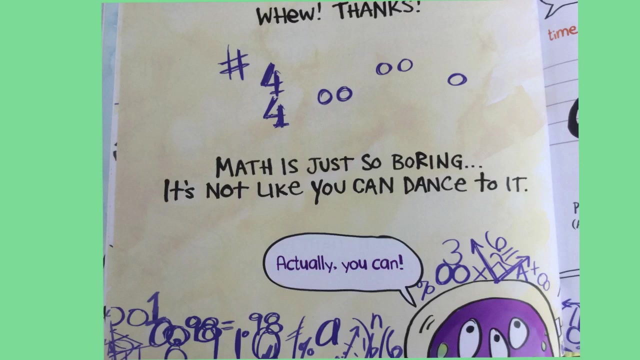 You got a little carried away. This is way too much math. Can we shake the book and make some of the numbers fall out? Just hold it tight and give a few good shakes. Woo thanks, Math is just so boring. It's not like you can dance to it. 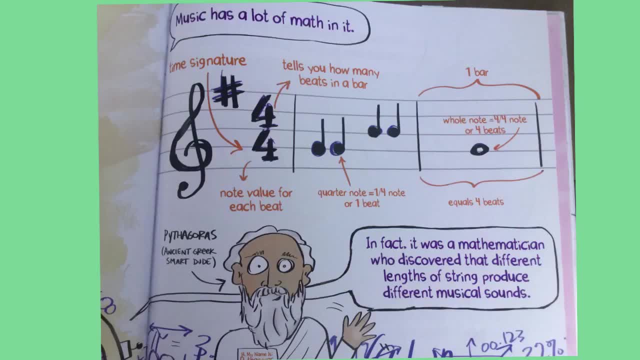 Actually you can. Music has a lot of math in it. In fact, it was a mathematician who discovered that different lengths of string produce different music, And that's why it's so important that you learn how to play the right notes. 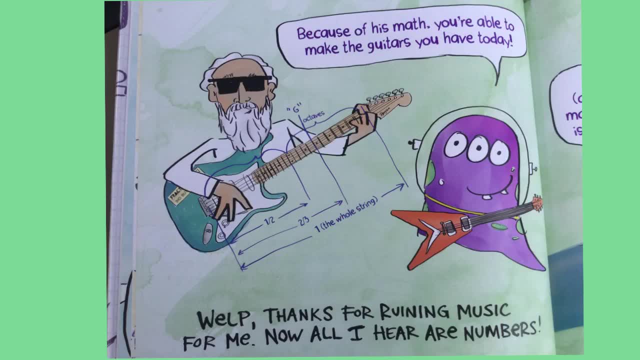 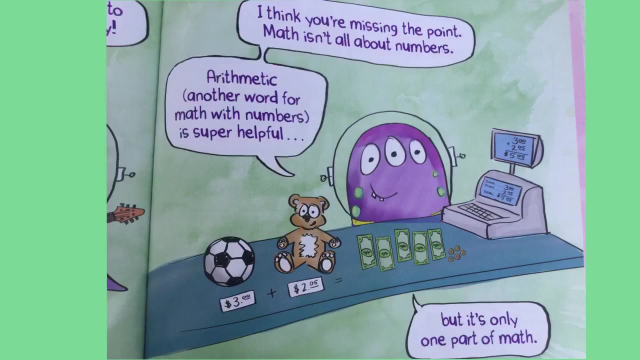 And that's why you learn how to play the right notes. Because of his math, you're able to make the guitars you have today. Well, thanks for ruining music for me. Now all I hear are numbers. I think you're missing the point. 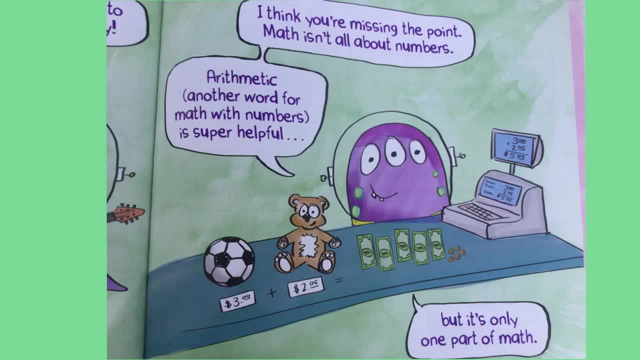 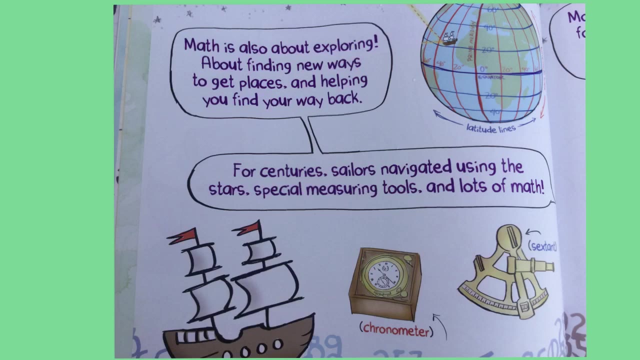 Math isn't all about numbers. Arithmetic- another word for numbers- is a very important part of math. Arithmetic is a very important part of math. Another word for math with numbers is super helpful, But it's only one part of math. Math is also about exploring. 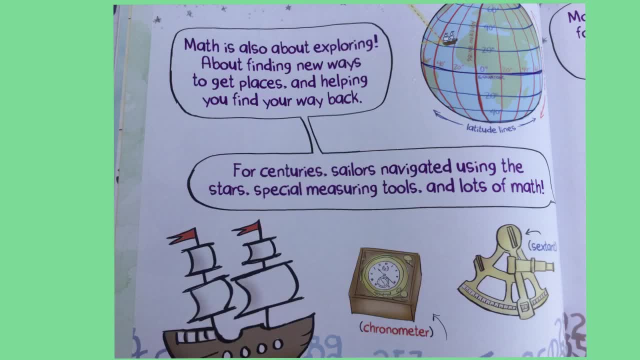 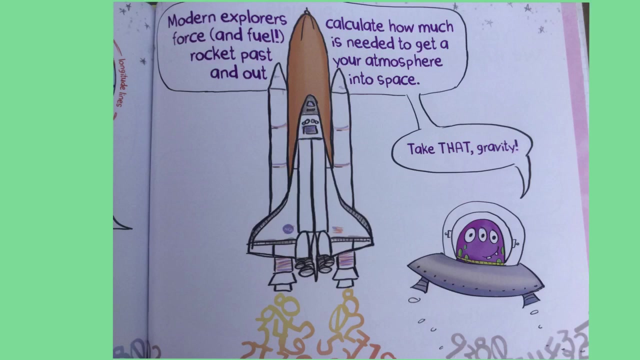 about finding new ways to get places and helping you find your way back. For centuries, sailors navigated using the stars, special measuring instruments, special measuring instruments and lots of math. Modern explorers calculate how much force and fuel is needed to get a rocket. 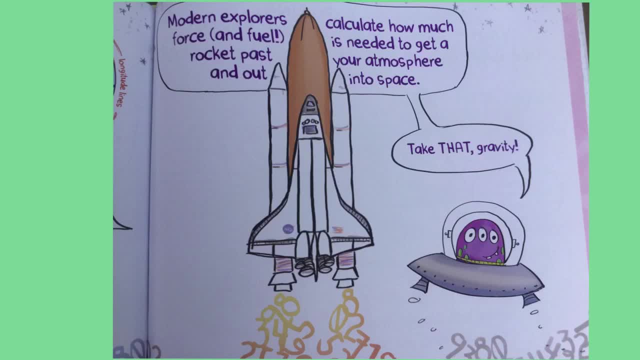 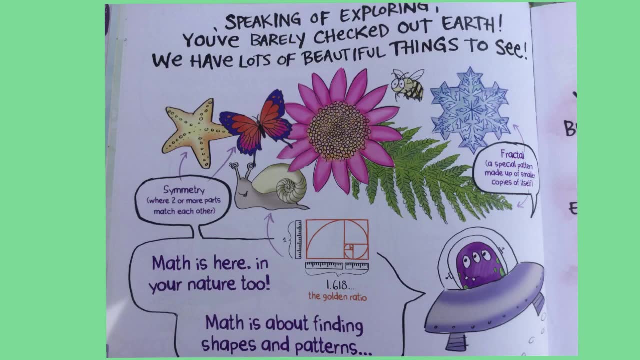 past your atmosphere and out into space, past your atmosphere and out into space. Take that gravity. Take that gravity. Speaking of exploring, you barely checked out Earth. You've barely checked out Earth. We have lots of beautiful things to see. 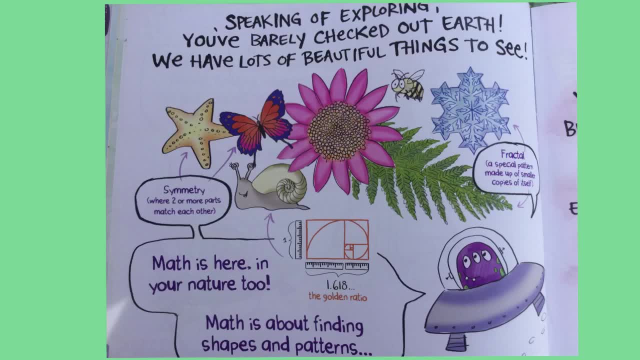 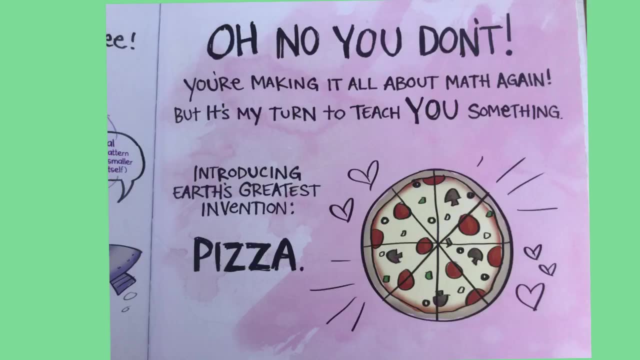 Math is here in your nature too. Math is about finding shapes and patterns. Oh no, you don't. You're making it all about math again, But it's my turn to teach you something Introducing the Earth's greatest invention: pizza. 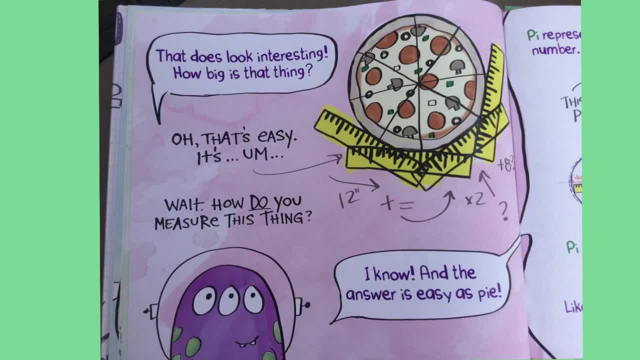 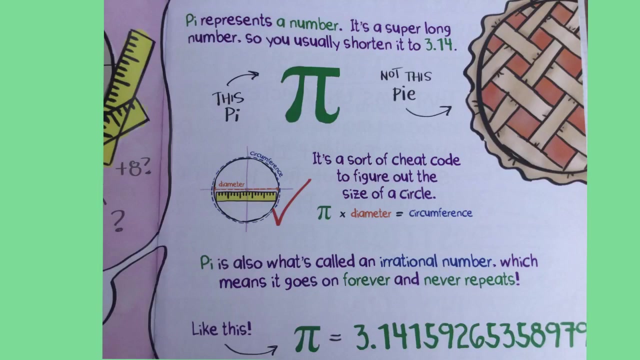 That does look interesting. How big is that thing? Oh, that's easy, It's um weight. How do you measure this thing? I know, and the answer is easy, as pie. Pie represents a number, It's a super long number. 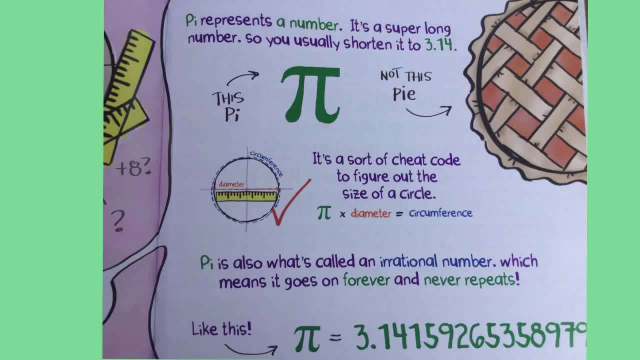 So you usually shorten it to 3.14.. It's a sort of cheat code to figure out the size of a circle. Pie times diameter equals circumference. Pie is also what's called an irrational number, which means it goes on forever and never repeats. 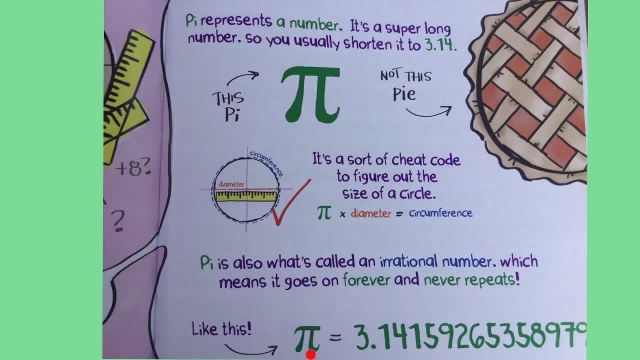 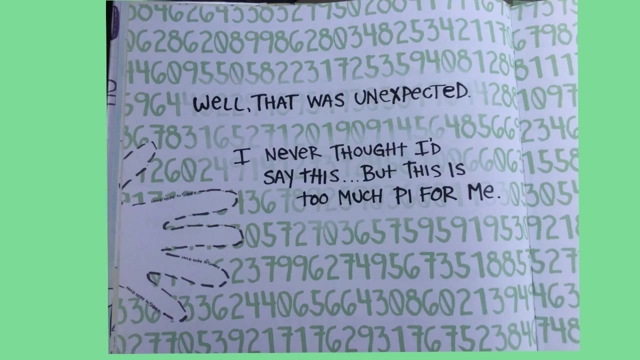 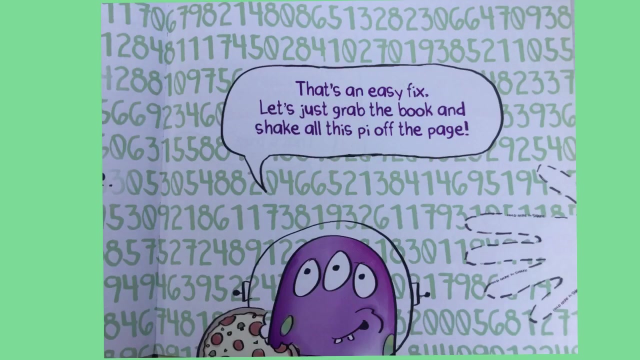 Like this Pie equals 3.14159265358979.. Well, that was unexpected. I never thought I'd say this, But this is too much pie for me. That's an easy fix. Let's just grab the book and shake all this pie off the page. 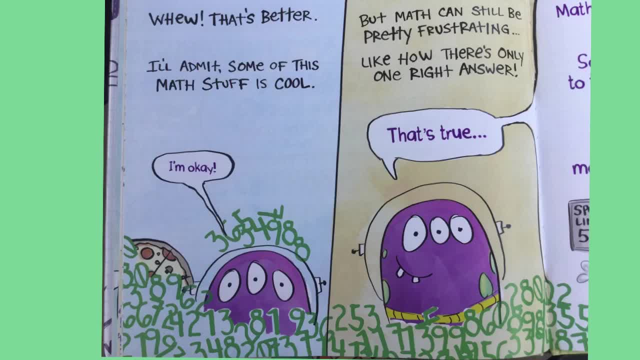 Woo, That's better. I'll admit, some of this math stuff is cool. I'm okay, But math can still be pretty frustrating, Like how there's only one right answer. That's right, That's right, That's right.